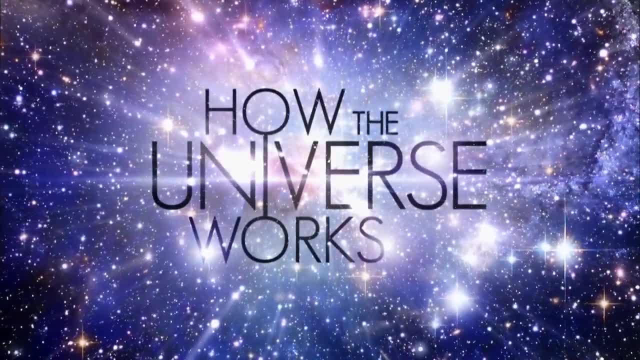 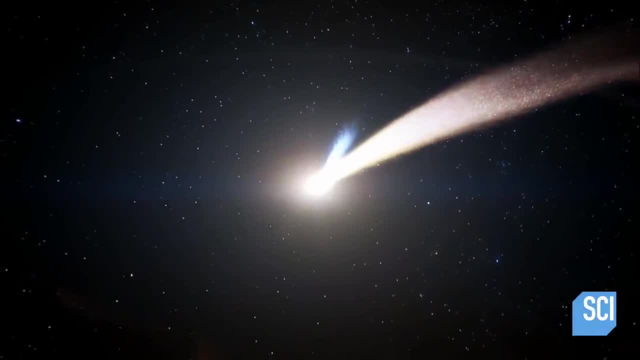 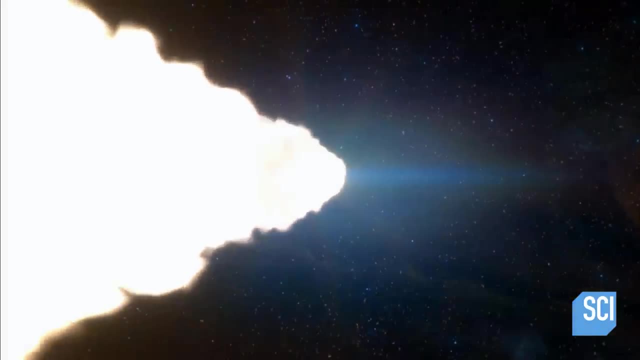 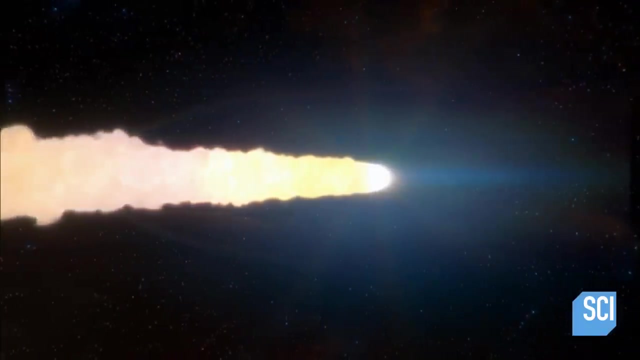 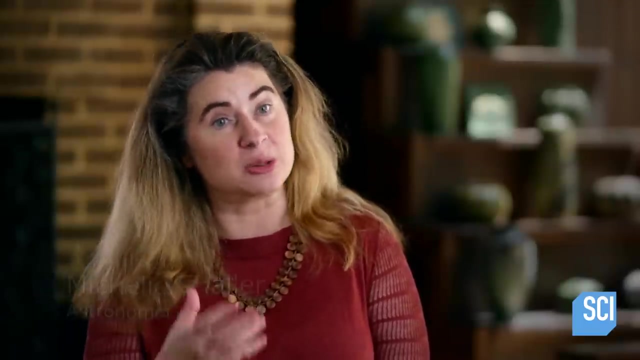 530 million miles from the sun, a tiny lump of ice and rock starts its journey towards the inner solar system. Scientifically, comets are more precious than pure gold. They are actual time capsules. They are preservations of what the chemistry, the environment was like when our solar system formed. 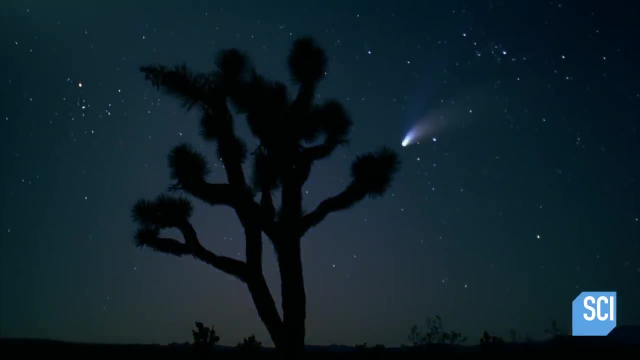 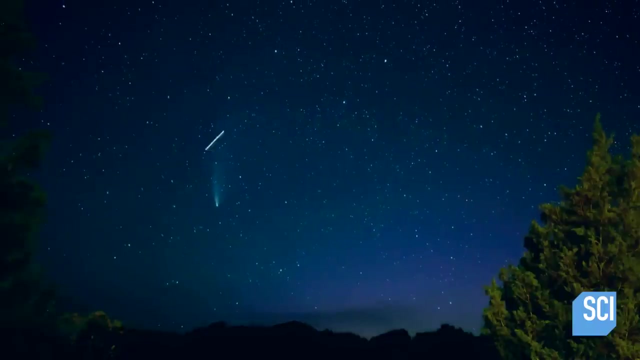 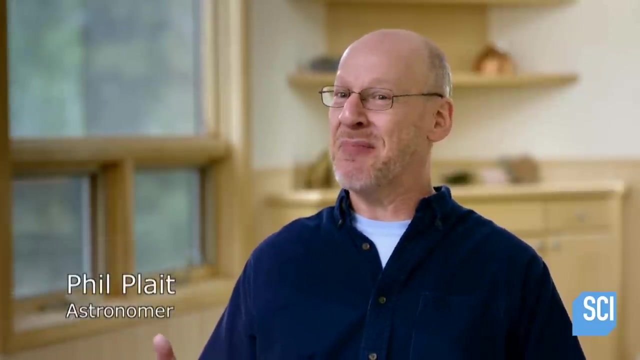 And they hold clues as to how our chemistry arrived here on Earth. Comets are some of the most valuable scientific treasures that exist. Finding a comet we can study is not an easy task. Finding the right comet for a mission, it's kind of like you're auditioning them, right. 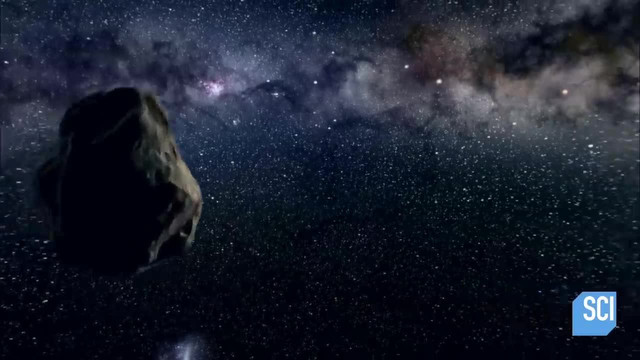 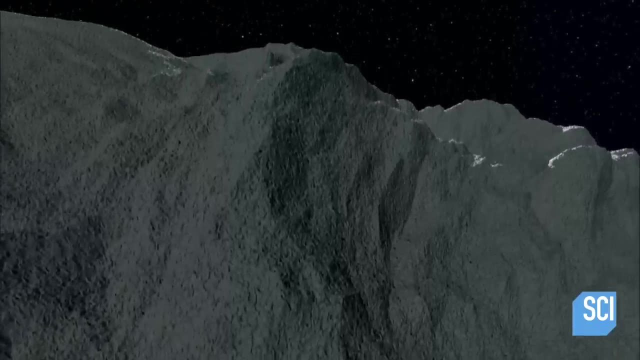 One comes in and it's like, oh, that orbit's okay, but it's not exactly what we're looking for. Oh, this one's too big, this one's too little, this one's too active. What we really want to see is that comet come from outer parts of the solar system. 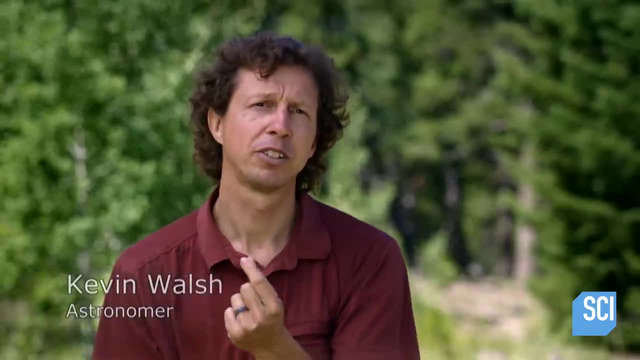 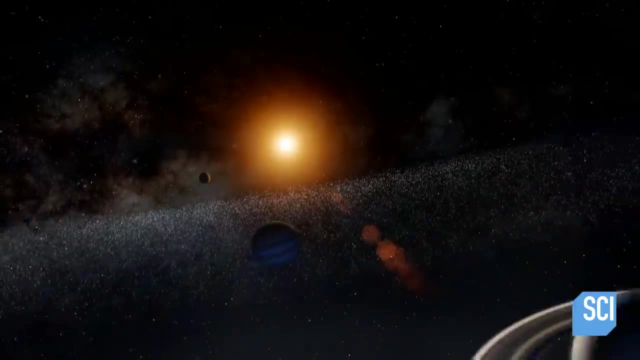 and get heated up as it gets close to the sun, pass around the sun and head back out to the outer part of the solar system. So you need to get way out in the solar system and catch a comet on its way in. Comet 67P fits the bill. 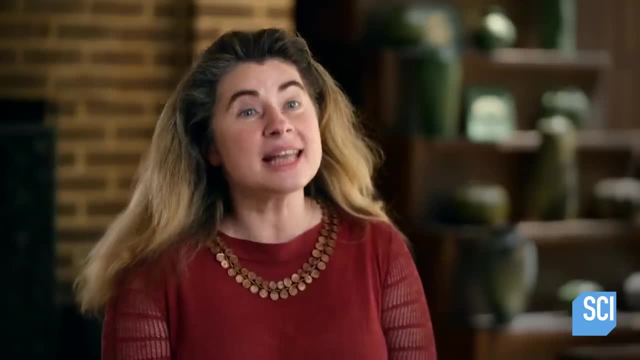 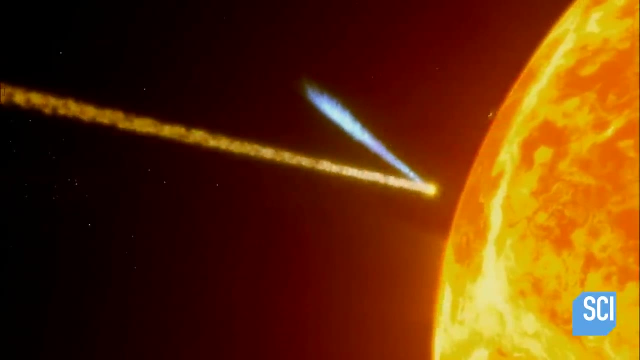 The special thing about Comet 67P is how accessible it is here on Earth. It actually orbits around the sun once every six and a half years, And its orbit doesn't take it all that far out- only about as far out as the planet Jupiter. 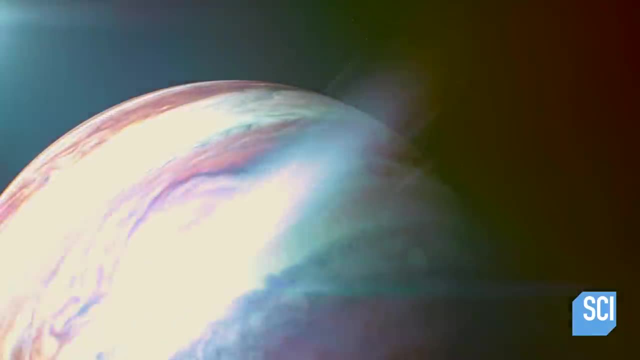 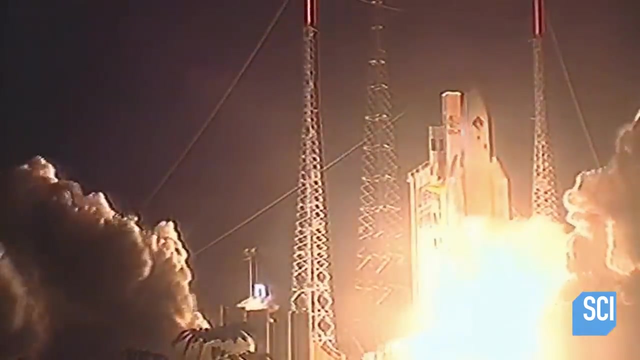 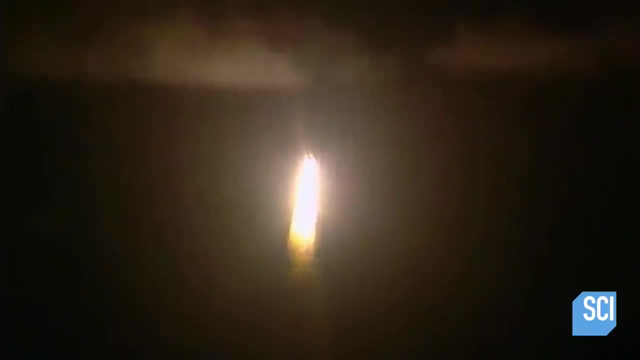 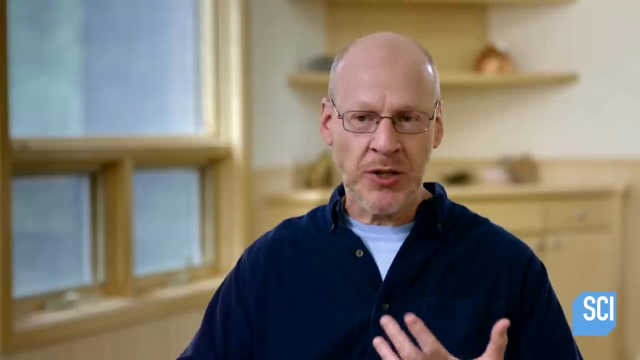 That gives us many chances to actually reach the comet and successfully rendezvous with it. 67P's moment in the spotlight arrived. The European Space Agency launched the groundbreaking Rosetta probe. For years we've studied comets from afar. We had never seen one up close with cutting-edge technology. 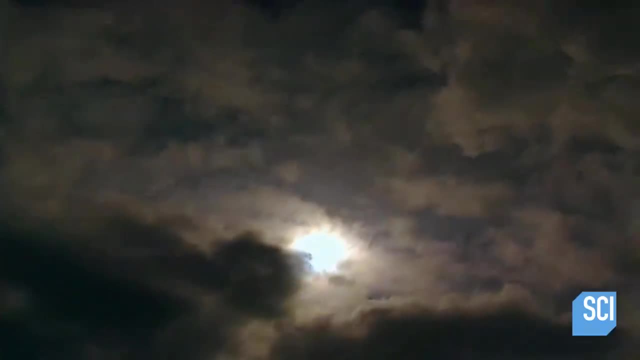 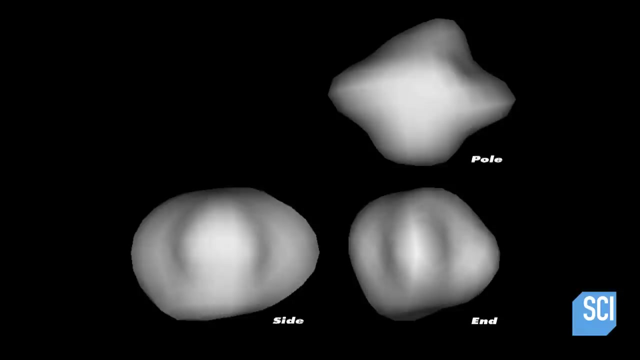 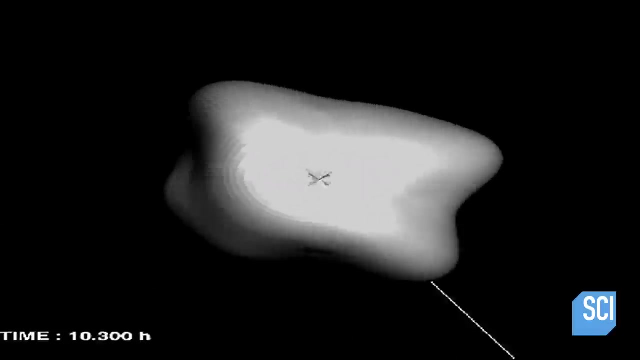 to learn about how comets behave as they orbit the sun. Missions to large planet-sized objects are hard. The Hubble Space Telescope's blurry images revealed Rosetta's target is just two miles wide. And not just a small target, a moving one. 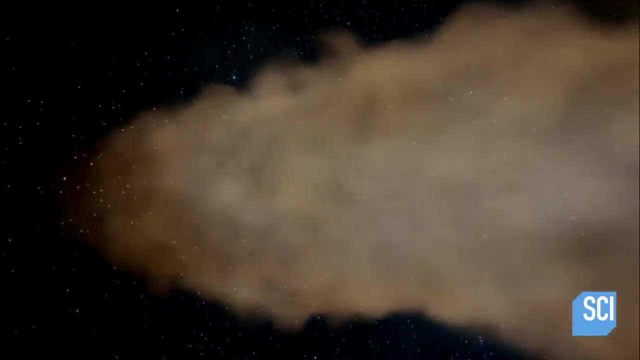 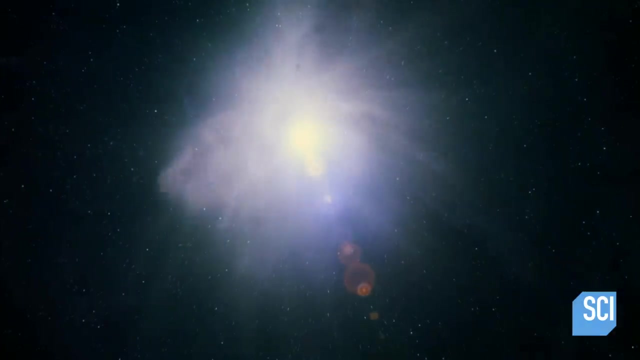 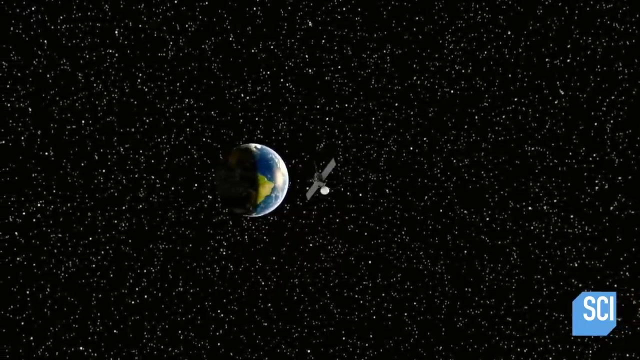 Comet 67P races through the solar system at over 33,000 miles an hour. The precision involved is pretty incredible. It's like making that hole-in-one golf shot from New York to San Francisco. But catching Comet 67P wasn't just a straight shot. 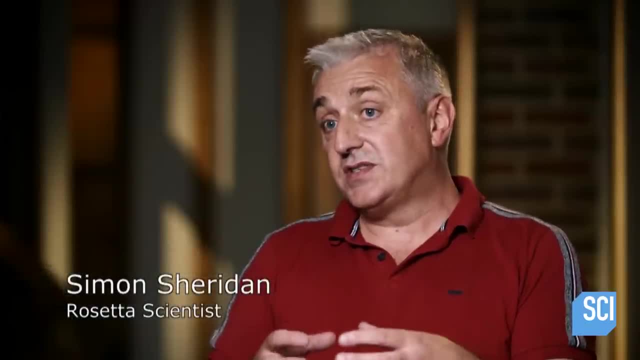 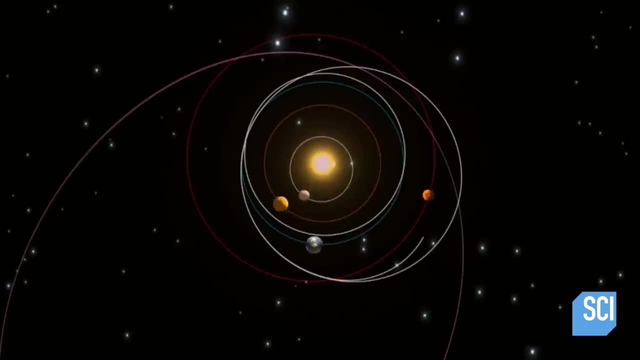 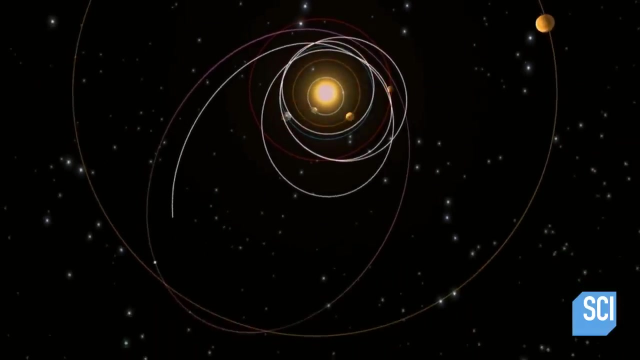 The spacecraft had to actually get the same sort of velocity as the comet, And with current propulsion systems we can't achieve that by flying directly to the comet. Instead, Rosetta performed a slingshot maneuver that would take 10 years. What it's doing is actually taking some energy away from the planet. 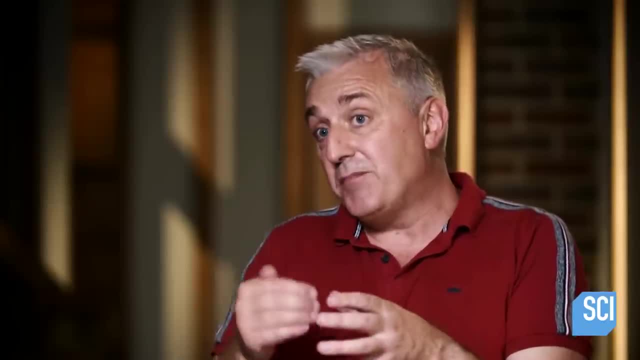 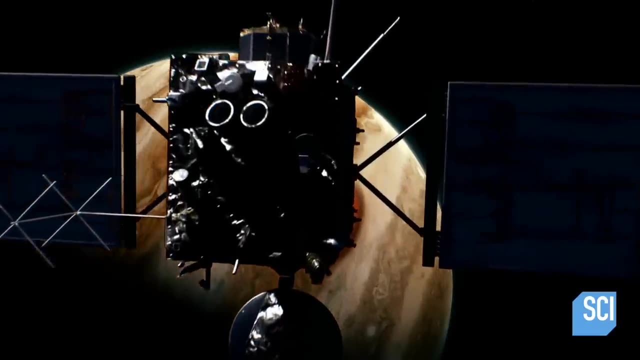 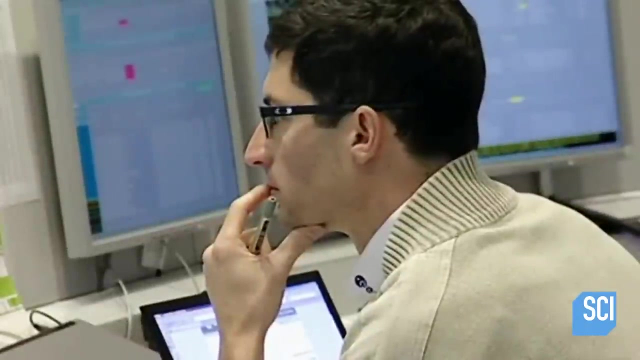 So it's slowing the planets down a little bit and then imparting that energy into the probe. Rosetta flew past Jupiter nearly 100 million miles from the warmth of the sun and entered the most dangerous part of its journey: hibernation. 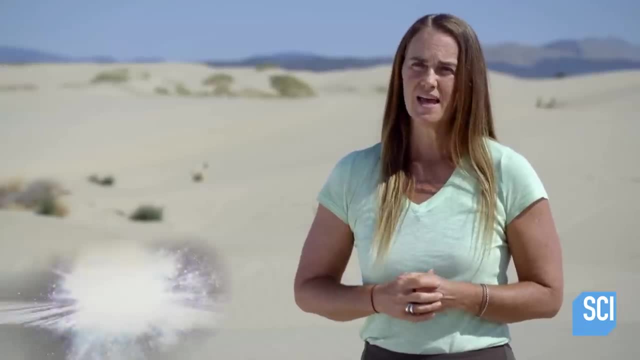 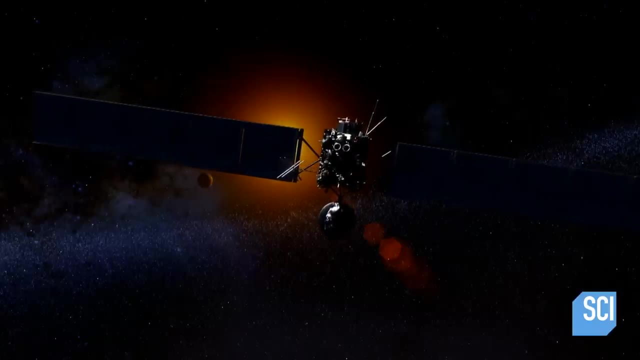 Even though Rosetta had solar panels on it, it still had to be put to sleep, And the reason for that is that it had to track 67P a ways away from the sun and there just was not enough collection area and solar power to be able to power the instruments. 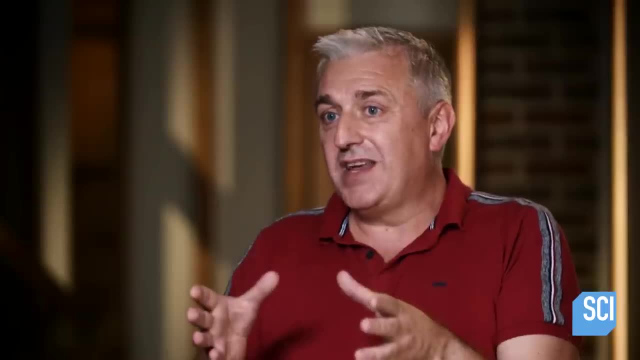 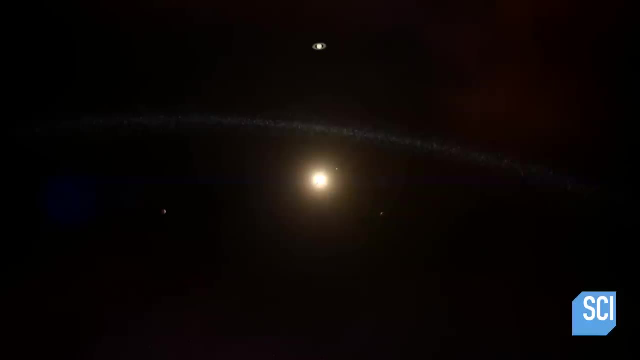 It's normal to put spacecraft into hibernation, But the worrying thing at the back of your mind is that it had never been done for this long before. 31 months of hibernation gave Rosetta's team plenty of time to worry about what could go wrong. 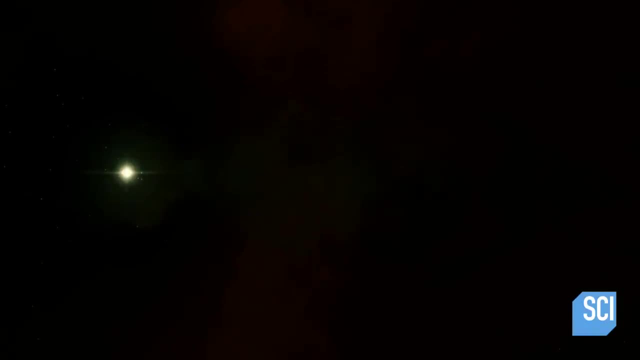 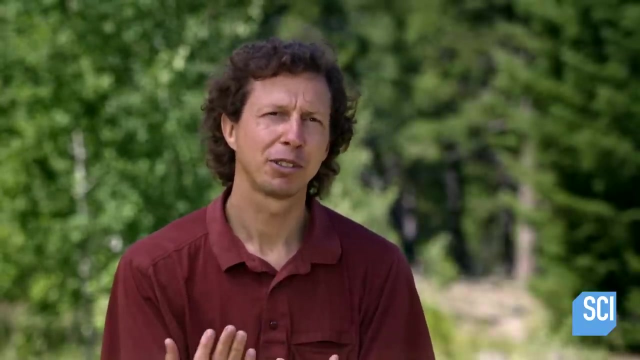 It's dark and cold out there in space. There's a lot of things going on, There's a lot of little micrometeorites out there And without the constant communication with that spacecraft it just is a little nerve-wracking when the day comes and it's time to flip the switch and turn it back on. 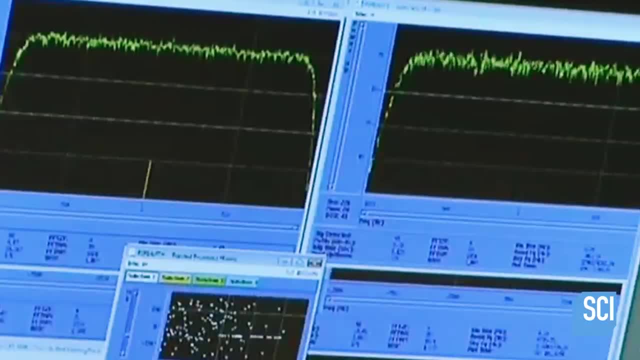 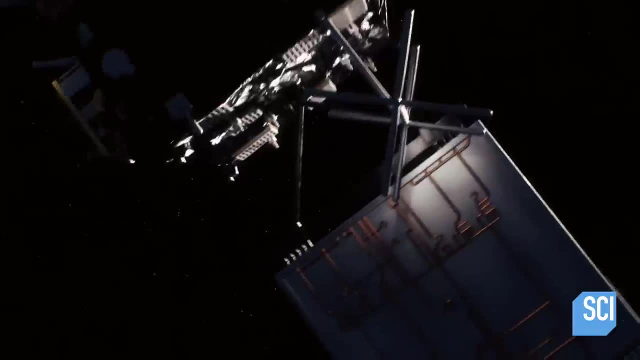 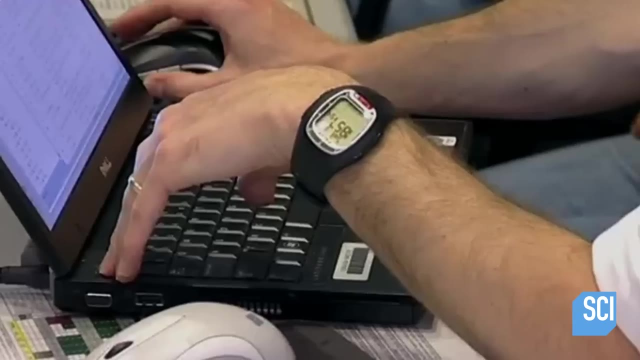 January 20, 2014.. After almost 10 years in space, it was finally time for Rosetta to wake up, reactivate its communication system and phone home. I mean, the tension was just palpable, It was just. I mean, how long do we have to wait before we're going to get the signal? 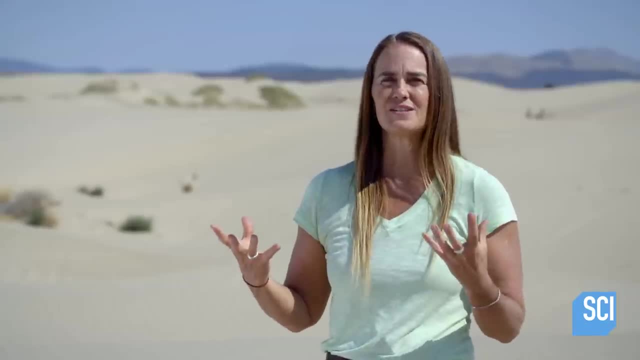 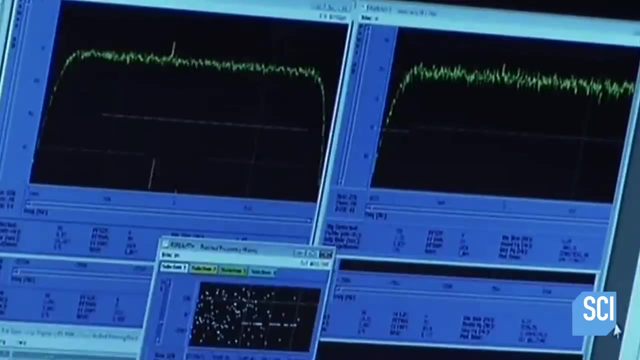 It's got to work. It has to work. Oh gosh, maybe it's just not going to turn on at all. Have we lost the spacecraft? And then the peak appeared on the graph. It's like, yes, we've got contact with the spacecraft. 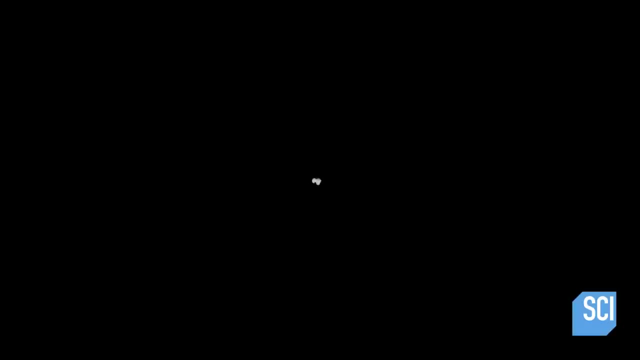 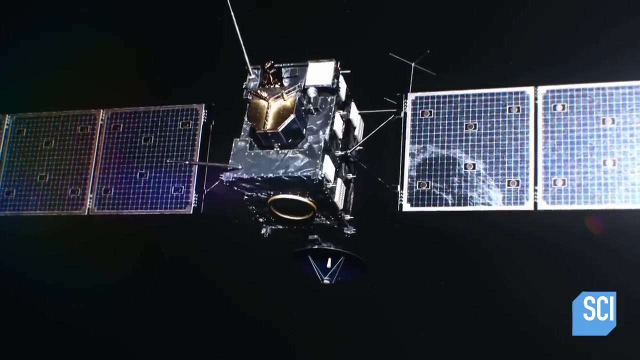 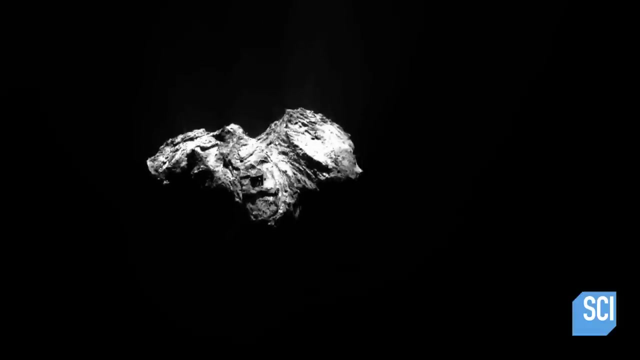 Rosetta began to send back images of its target And, after months of seeing a small dot in the distance, the comet slowly came into focus. When I first saw Rosetta, when I saw this comet crystal clear, this mountain floating in space of ice and rock, 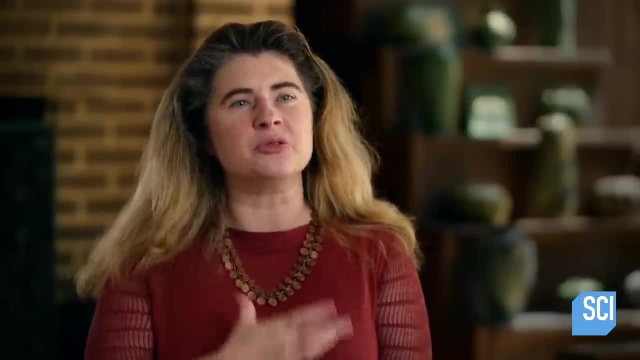 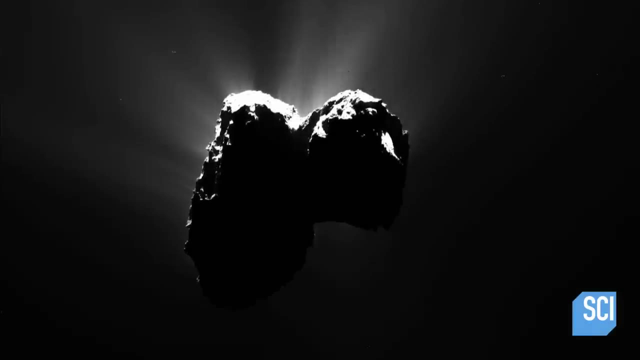 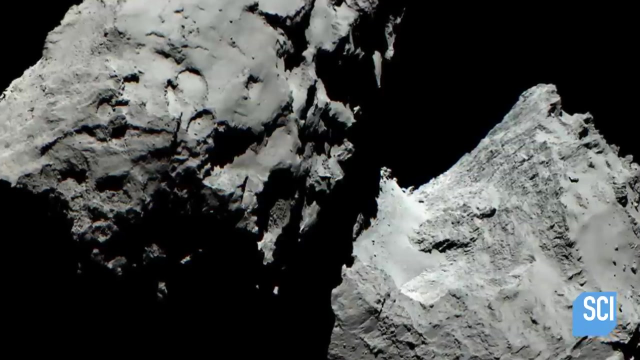 my heart just dropped. They were some of the most dramatic, beautiful images I have ever seen. And then, as it got closer and we got to see more and more details on it- yeah, that's when things started getting really strange. Quite simply: arrival at 67P. 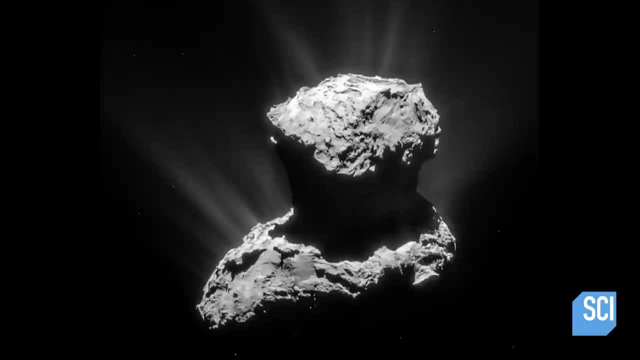 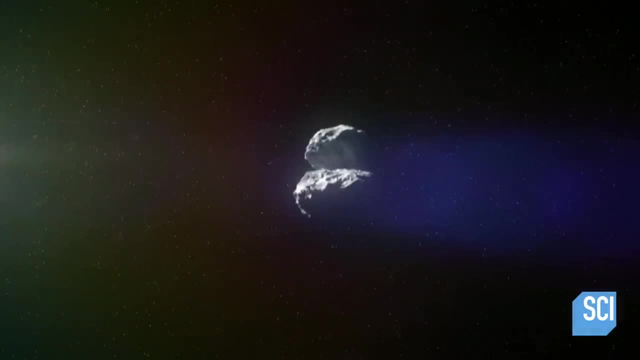 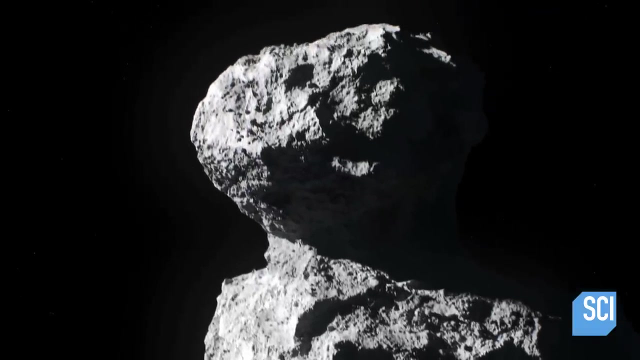 we expected to see something shaped like a potato and we found something shaped like a rubber duck. 67P is no ugly duckling, but its strange shape created a problem for Rosetta. Orbiting the comet was going to be far more difficult than anyone had imagined. A planet has a lot of gravity, so you can send the spacecraft out there and then just slow it down a little bit with a rocket burn and it'll drop into orbit. In the case of Comet 67P, you're dealing with a very small little rock. 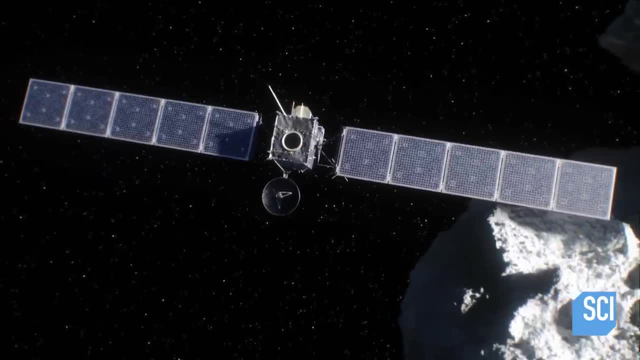 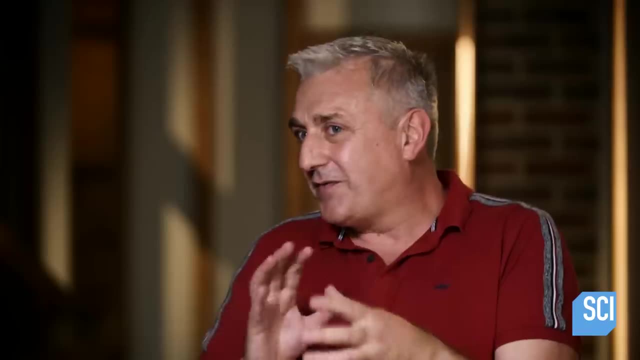 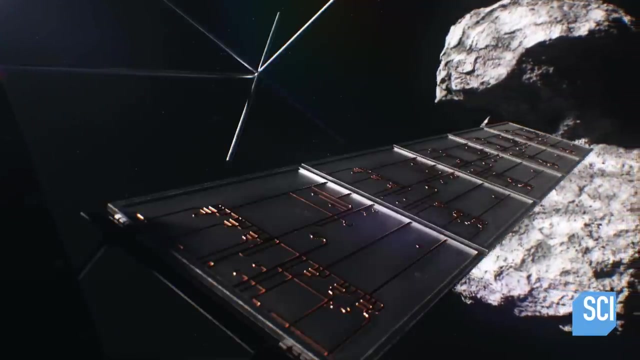 The spacecraft cannot feel the gravity of that rock, at least not until it's right up against it. The engineers had to actually plot triangular orbits. It was a very complicated set of maneuvers. Once in orbit, Rosetta could start work- Its first task. 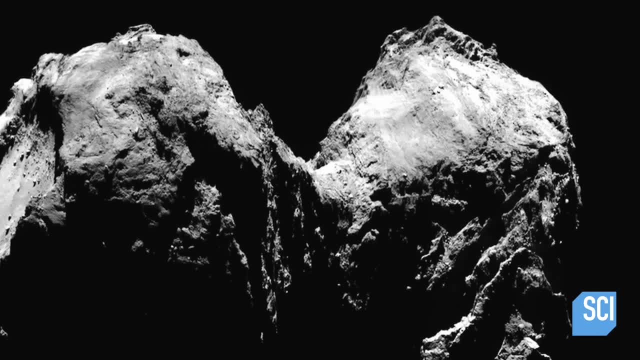 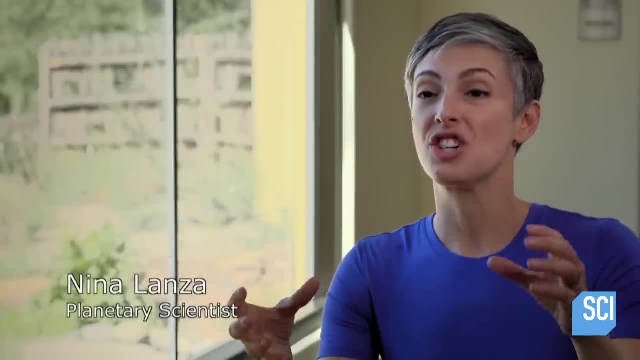 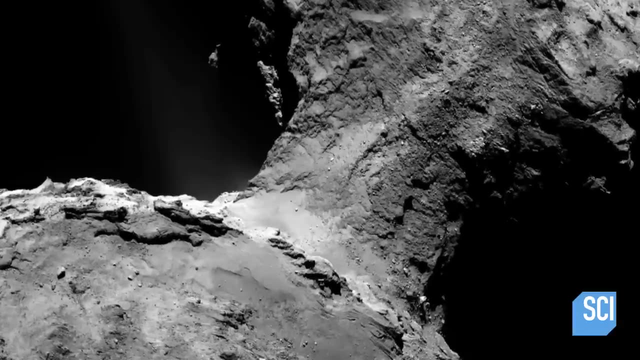 Figure out how 67P formed. So how did this comet get this weird shape? There's two main ideas. One is just that it was eroded somehow in the center, and so it started off as a more spherical thing and became the shape it is today through some unknown process. The other idea is that it started as two separate objects. Space rocks normally hit each other hard. They collide with an average impact speed of more than 11,000 miles an hour. That's five times faster than a rifle bullet. Was 67P involved in a pileup? 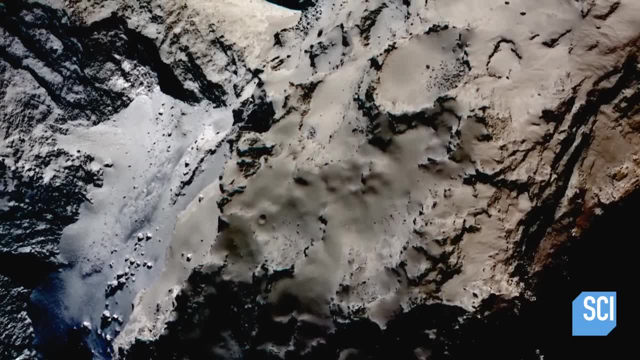 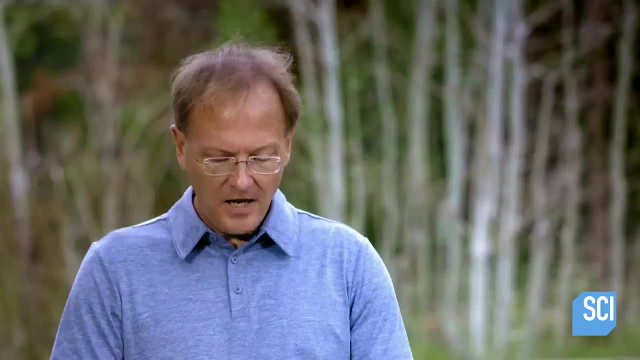 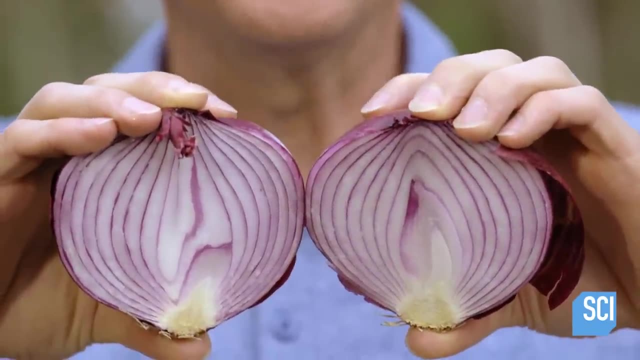 A clue came from the distinct layers on the comet's surface. The layers in Comet 67P are a little like the layers in an onion. If you see them aligned, that's a clue that perhaps the object formed as a single entity and only eroded later into its present form.